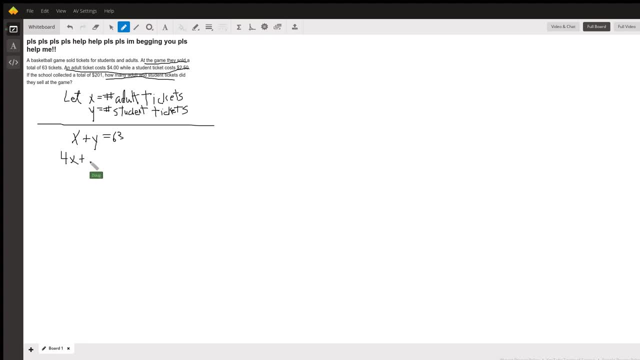 ticket- student ticket- brings in two dollars and 50 cents, And I'll just write that as 2.5.. And that brings in how many dollars? What does it say? 201 dollars. Okay, now, at this point you have what's called a system of two equations and two unknowns. 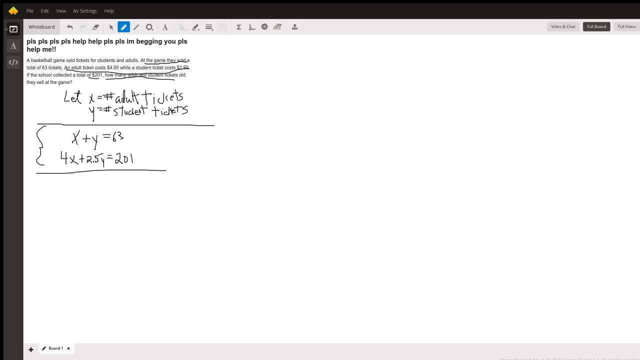 You can use the addition elimination method, You can use the substitution method. When it's easy to solve for one variable, I like to use the substitution method. So here I'm going to solve for y. y equals 63 minus x Subtract x from both sides. Now I'm going to take this expression: 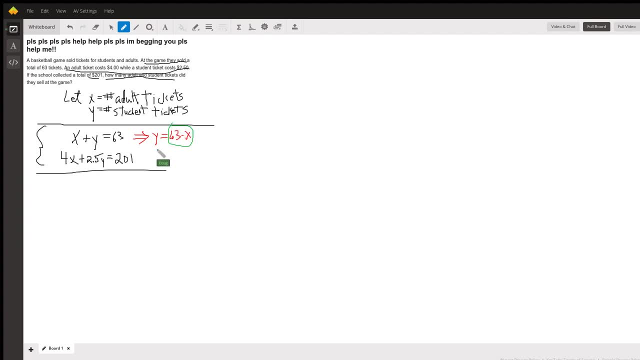 which is equivalent to y, and substitute it into the other equation. So my new equation is 4x plus 2.5 times 63 minus x. That's what y is. That has to equal 201.. Now how you want to solve for x at this point. 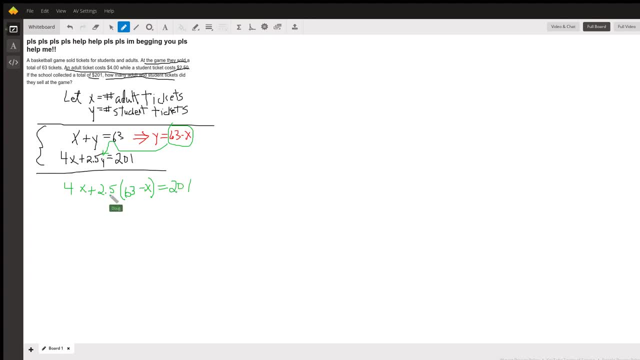 you might want to clear the equation of decimals by multiplying every two, three, four, five, six decimals by multiplying every term by 10, which is what I would probably do, since I don't like to work with decimals. So I'd get something like 40x plus 25 times the quantity 63 minus x. 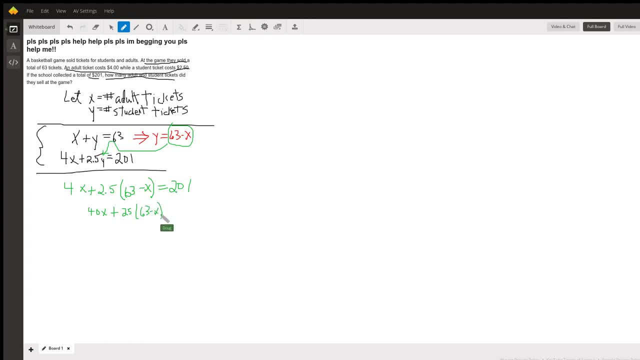 equals 2010.. I multiplied every term by 10 just to get rid of that decimal. I'll let you take it from there. So I'm going to repeat this: 25, combine similar terms and solve for x, And that'll be the number. 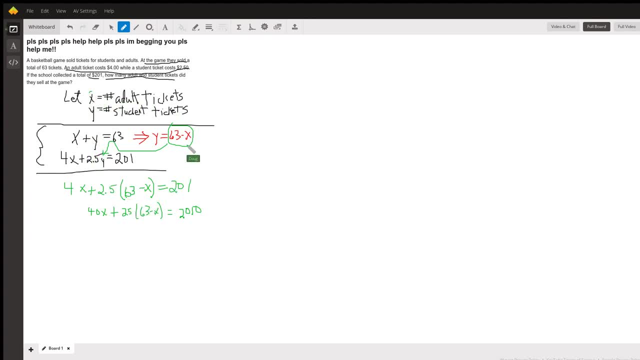 of adult tickets. Then, when you get x, substitute that number in here and you'll get y. Okay, there you go. Hope that helped. If you have any questions, post a comment.